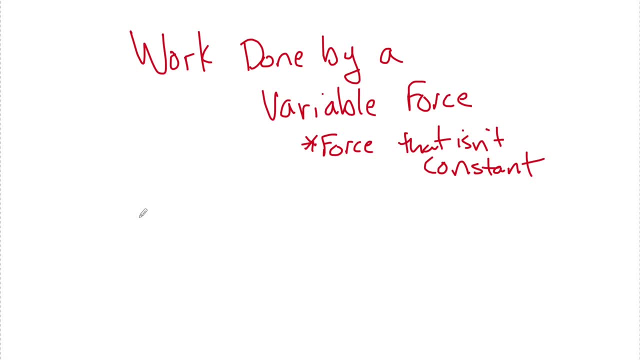 necessarily need calculus, But we're essentially going to do this by using a F versus X graph. Okay, so let me just show you how we're going to do that real quick. First, let's talk. let's just look at. first, a constant force, All right, so if we could use this graph, if I had a graph. 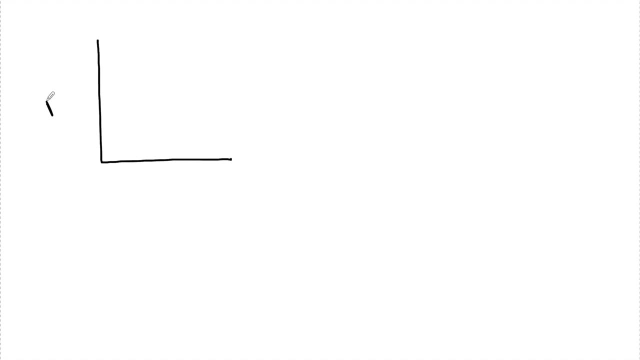 that looked like this and we'll say that this is F over here and this is the displacement over here. in meters we have 1,, 2,, 3,, 4, 5, 6,: 1,, 2,, 3,, 4,, 5, 6.. 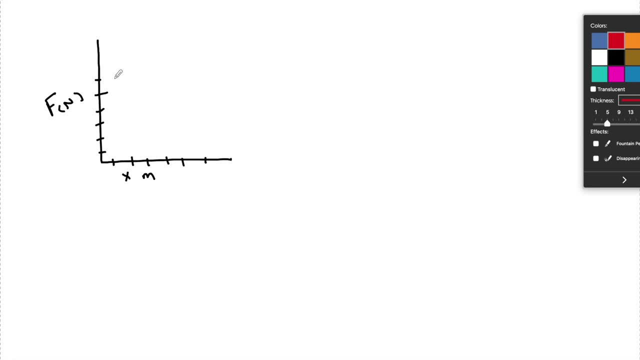 If I said that there is a force, okay, was applied to a box over this amount of time and I can ask what is the work done on the box? Now, because this is very easy and we know that work is equal to F times X, I can ask what is the work done on the box? 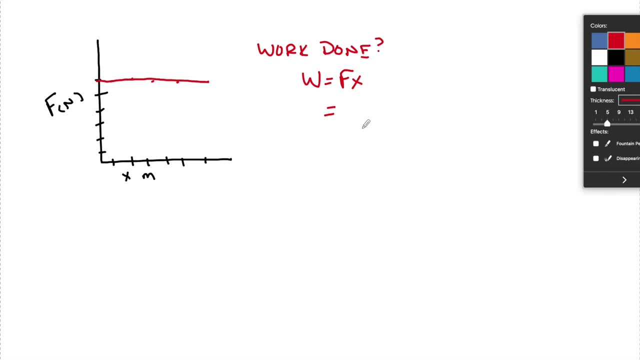 I can say: well, at every single moment on this graph, the force is constant. okay, It was 6 newtons and it did that over 6 meters. Therefore, the work done was 36 joules. okay, So that's like. 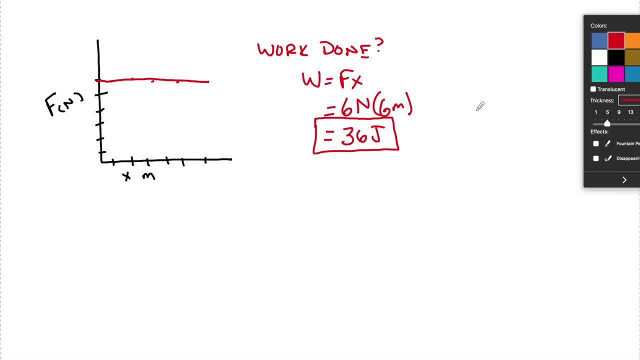 the mathematical way that we solve when the work is constant. But one thing we never really talked about which we could do is we could find the area under this curve. Even though it's a straight line, we still call it a curve, right. 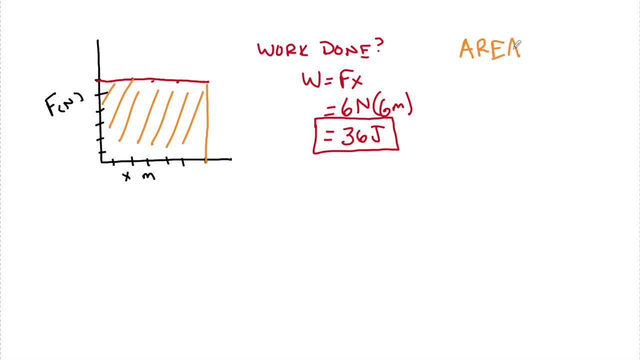 And the way we're going to do that is, when we find area, it's just going to be base times height in this situation. So the base was 6 meters, the height was 6 newtons. Therefore, the area told us that the work done was 36 joules. okay, Super easy when we have a nice constant velocity. 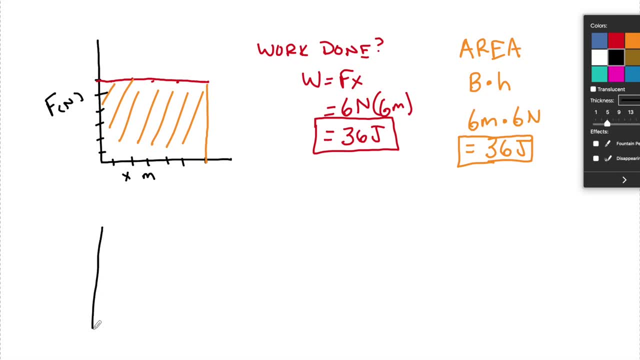 Well, what happens when that force varies a little bit and we have F of newtons again and we have X in meters 1,, 2,, 3,, 4,, 5, 6, 1,, 2,, 3,, 4,, 5, 6.. We come out here to 0.66,.